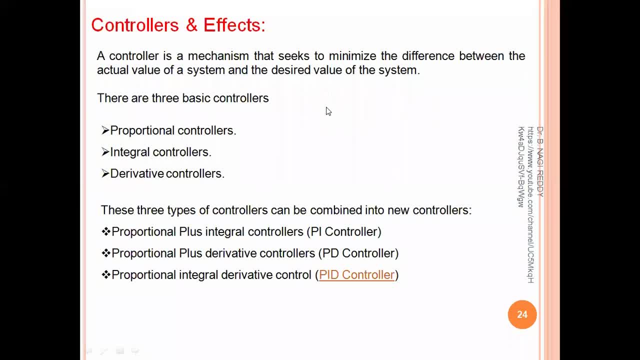 So that is the general meaning of a controller And basically there are three types of controllers. Basically, there are only three types of controllers. First one is a proportional controller, simply called as a P-controller, And the second one is integral controller, simply called as I-controller. 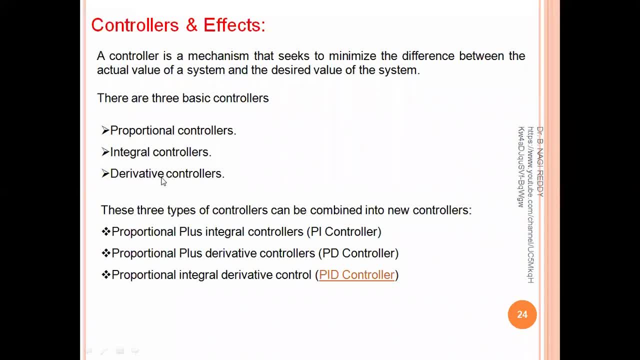 The third one is derivative or differentiator. Derivative, Derivative or differentiator controller, simply D-controller. So P, I and D are the three basic controllers. So actually this controller is included to our main plant of the system in order to reduce the error difference. 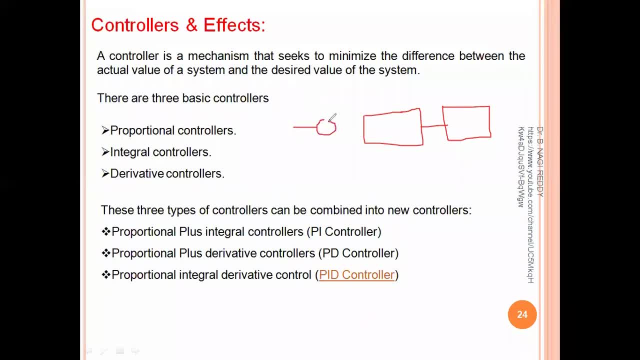 In order to reduce the error difference between the actual Actually input to the feedback signal. So this is the rough diagram of a typical closed loop control system. So this is a typical closed loop control system. Here we have input generally R of S. 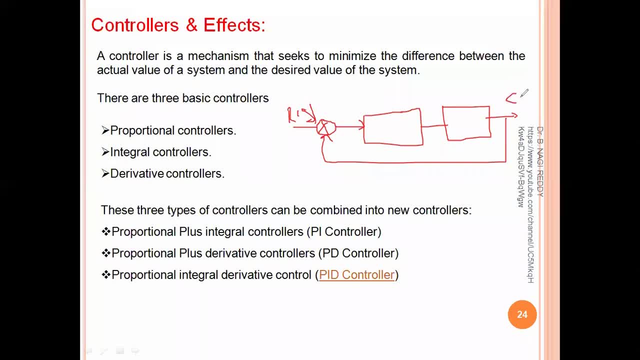 And we will have a output which is C of S Right And this is our feedback back and this is our complete plant transfer function. g or gc complete transfer function, or simply we may call this as open loop transfer function. this is open loop transfer functions. 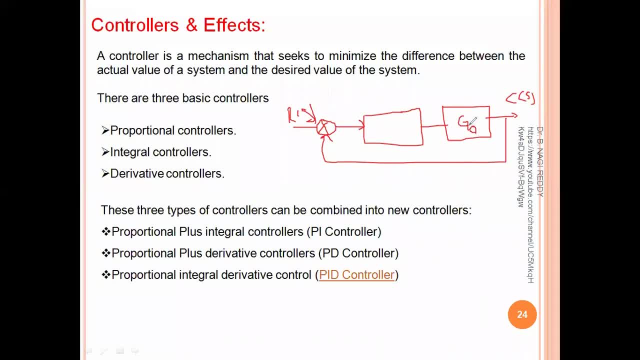 g naught. you can say you can, you can use any any term. so g naught is the open loop transfer function. then what about this block? this block is the controller. so this block, what it will do is, before of this block, we will have the error signal right. 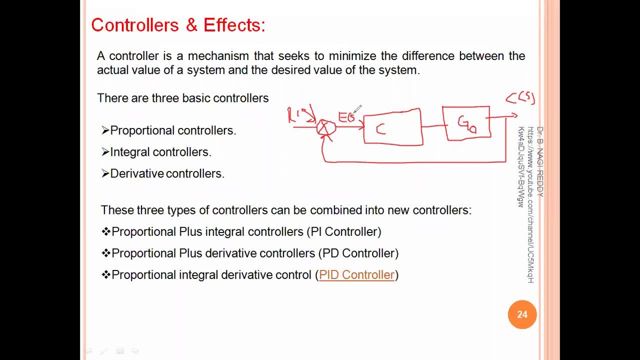 so this error signal is regulated by this controller and this controller produces a control signal here to band open loop gain. by sending this control signal to the controller and this controller will send a control signal to the controller, this plant will work properly. that means this entire system will work properly. 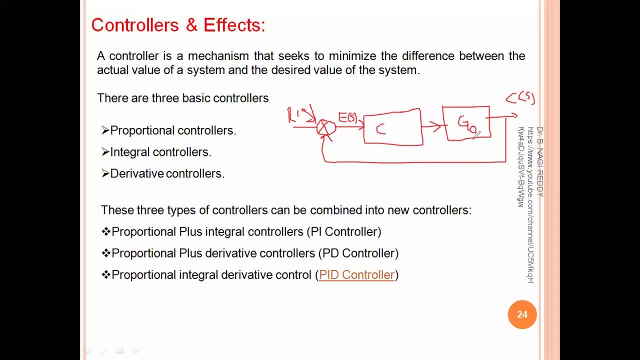 so because of this controller, we can control this plant effectively. so what this controller will do is it will take the error signal and it regulates this error signal and produces a control cell. this control signal helps the plant to work properly. so this is how a general concept, general block diagram, representation of 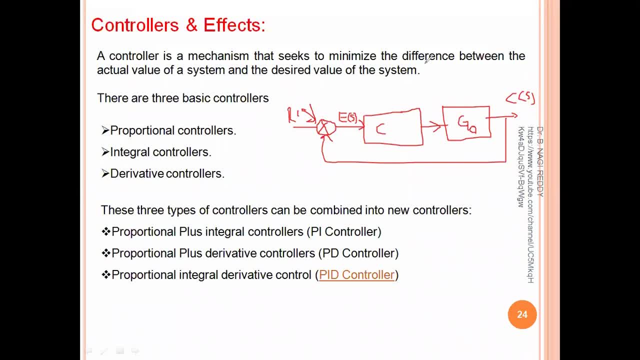 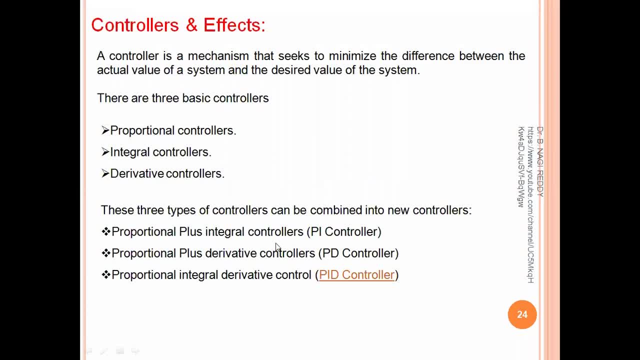 another three types of controllers, namely proportional plus integral controller. simply we call pi controller. so this proportional and this integral control, these two will be added together to get this control. what is that? proportional plus integral? so we need to add proportional controller along with the integral controller to get this combination and the second combination. 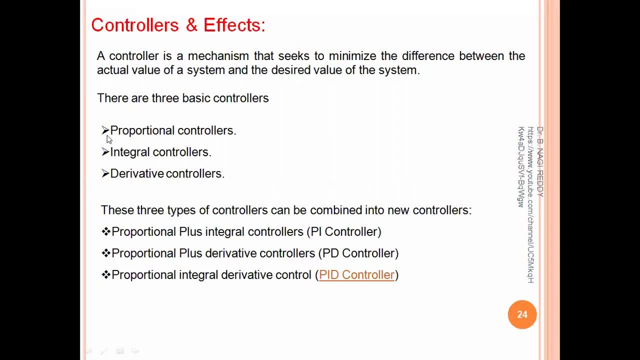 is proportional plus a derivative, so p and i, and the second combination is p and d. see, obviously, in each and every controller, proportional controller must be there because, because of the nature of proportional controller, we have to use proportional controller each and every combination. that's why you can see all these three combinations. you will find the proportional. 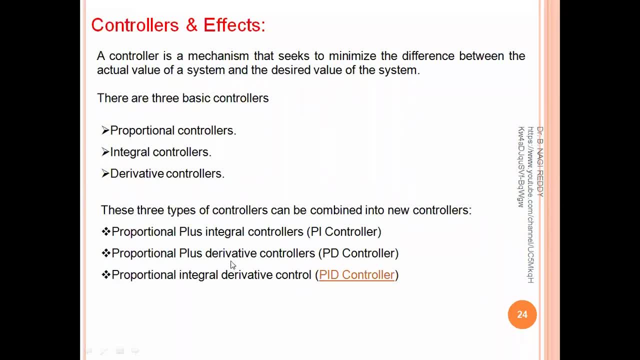 controller. so the second combination is proportional plus a derivative, so p and i. and the second combination is p and d type, includes proportional with derivative, which is simply called as a PD controller. And the third one is combination of three, which is proportional, integral derivative types. So 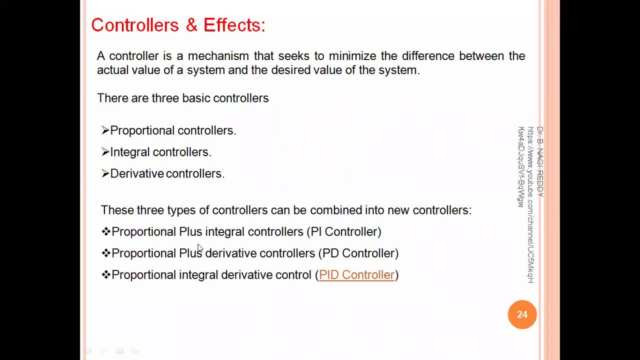 this is very important: PID controller and PA controller. these two are very much important in the projects point of view or in the what in the R&D point of view, because whenever we design a controller, these are the basic combinations. these are the basic utilized, most utilized. 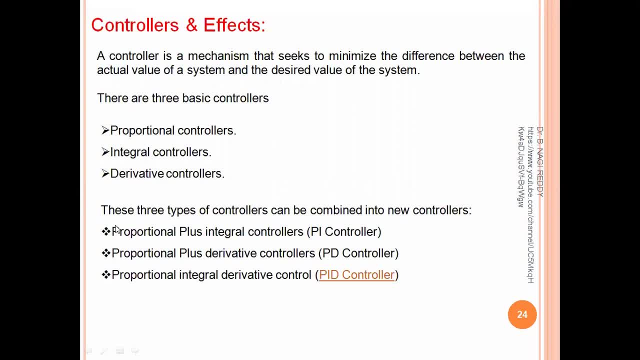 basic controls. These are the most utilized the basic controls In today generations. also, these controllers are very much competitive for the most of the advanced control techniques. Okay, so totally, we are having six controllers: three are basic and three are combination. 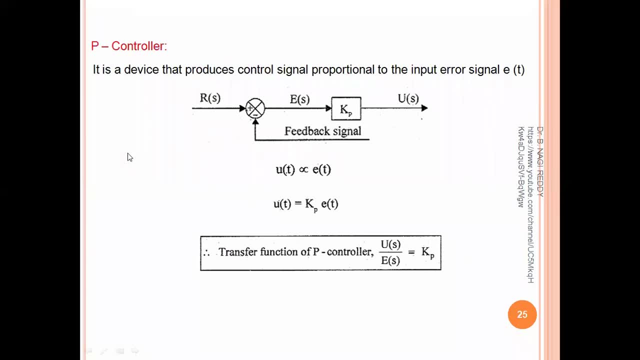 Let's see individually The first one, which is P controller. Now you can see here the P controller. what it will do is P means proportional right. So what it will do is it produces the control signal, which is the control signal means U of S. 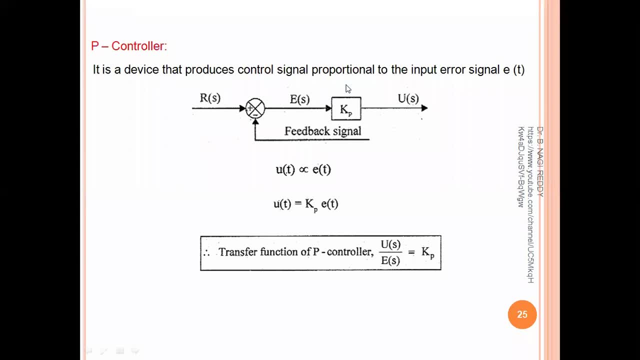 So U of S is the control signal here. So it produces the control signal which is proportional, Proportional to the error signal. So E of S is the error signal in Laplace domain or in time domain. we can represent it as E of t, small e of t. you know that, small letters. 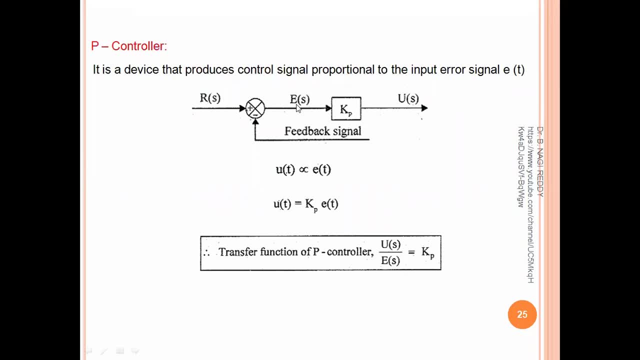 represent in time shows the time domain. capital letters shows it is in Laplace domain. So what it will do is it will generate a control signal U of S which is proportional to the errors. That's the control signal. That's why it is proportional. the generated control signal is: 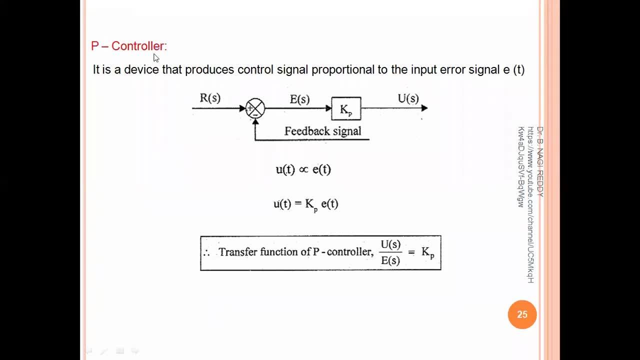 proportional to the error signal. That's why this controller is called as proportional controller And by this definition we can write in a time domain. if you want to write that in time domain, U of t is the control signal in time domain and E of t is the error. 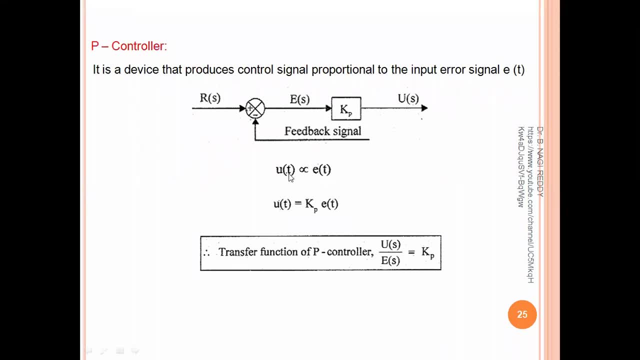 signal in time domain. So according to the definition, the control signal must be proportional to the error signal. So in order to eliminate this proportionality, we use a constant that is Kp. This constant is called proportional constant or simply gain of the p system. 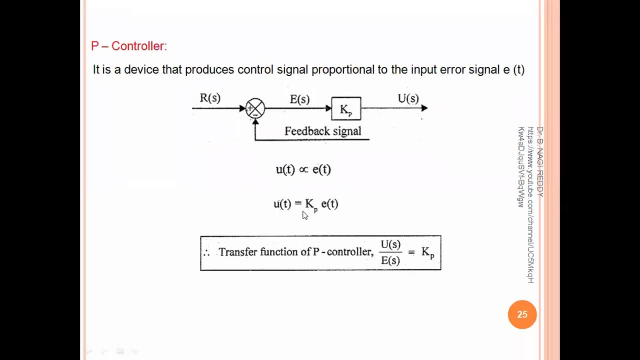 Proportional controller, gain of the proportional controller, And if we apply Laplace transforms to this, we can get the transfer function of this particular controller. What is the transfer function? If we apply Laplace transform to this, U of S and here it will be E of S. So output is U of S, input is E of S. 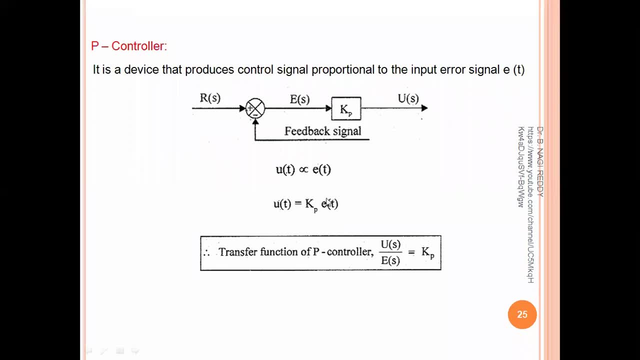 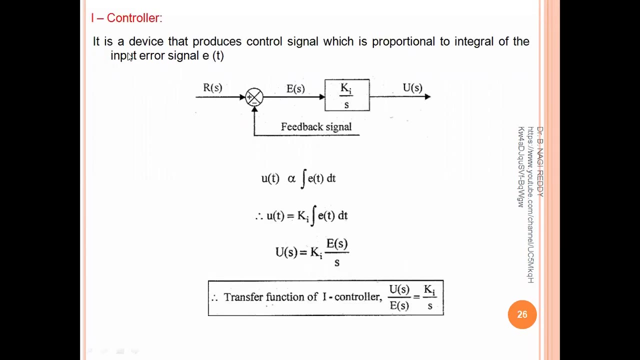 So the transfer function will be U of S by E of S, U of S by E of S, which is Kp. So this is the gain of this particular p controller. Right Coming to the I controller, the I controller is nothing but the integral controller. Integral means integration. 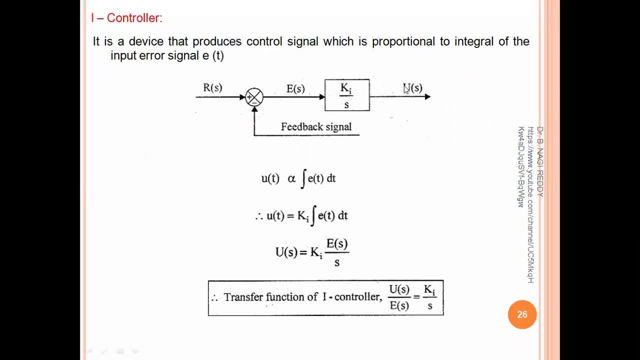 So this produces the control signal. that means U of S which is proportional to integral of the input error signal. So the produced control signal is proportional to integral. So we need to do the integration to the error signal to get the output. So from this definition we can write: U of T is directly proportional to integration of E of T. 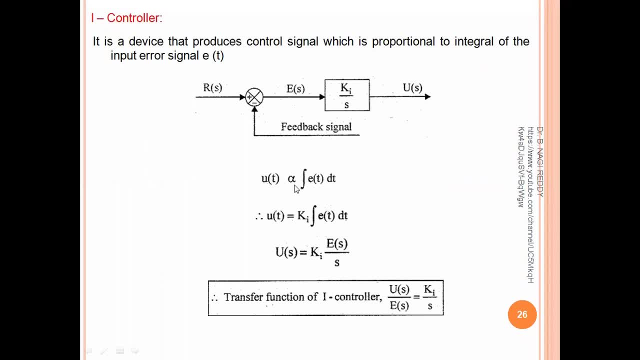 E means error, U means control signal. So the control signal is directly proportional to integral of error signal. Okay, So in order to eliminate that proportionality, we use Ki, which is integral gain. Simply, we call as integral gain Sometimes. 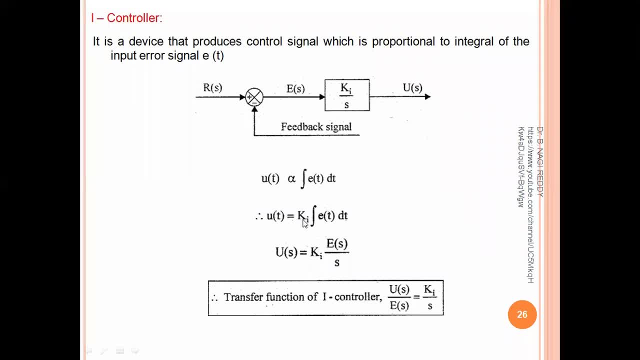 we may write this: Ki as Kp by Ti, Kp by Ti. Kp is the proportionality constant which we seen in the last concept Ti. Ti is the integral time constant, So Kp by Ti is Ki. We can write like this also: Ki can be represented in the proportionality constant. 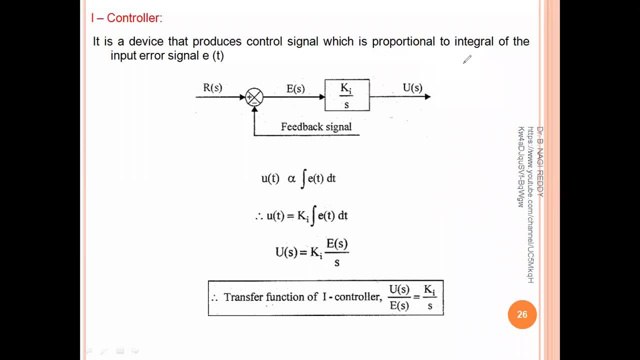 In this manner. Okay, So in a similar way, what we have done for the P controller, we can do here also. So what we can do, just simply use Ki in the place of proportionality and then apply the Laplace transforms. Then we will get U of S is equal to Ki into. 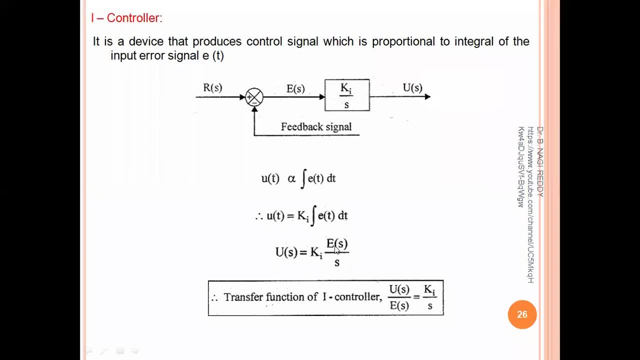 See, here we are having first order integration, So we'll have 1 by S according to Laplace principle. So for this we can write the transfer function, which is U of S, by E of S, because U of S, which is control signal, is our output, E of S, error signal, is our input. So U of S by E of S will be. 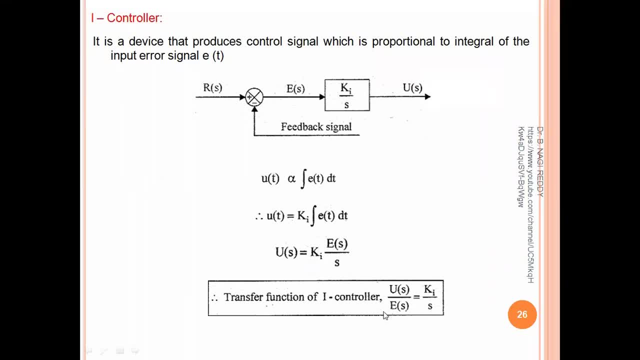 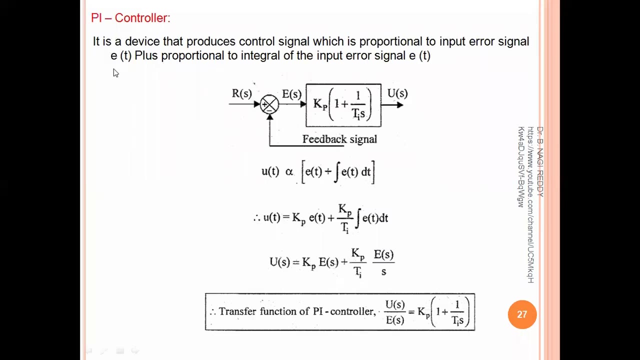 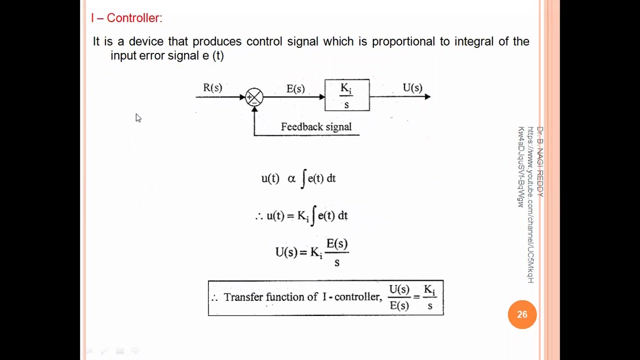 Ki by S. So this is the transfer function of our integral controller. Here we have to do the controller is called as integral. similarly the derivative control, also the same. here. if you want to write the derivative controller individually, we will have by dt. here d e by dt and we will get. 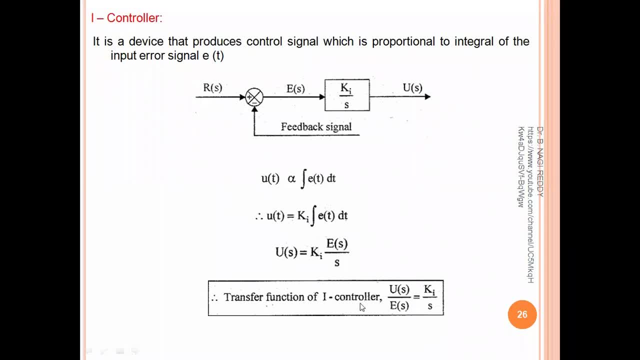 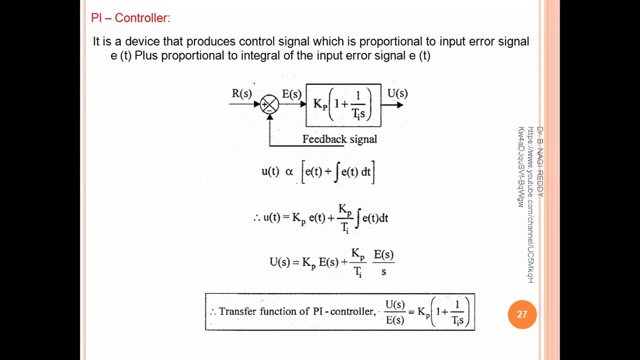 s here. so in the same process we can also calculate the transfer function for the derivative controller also, but independently. the derivative controller doesn't have much importance. because of their drawbacks- we'll discuss that later. what are the drawbacks of individual derivative controller and all and the first combination, which is p i controller? so what? 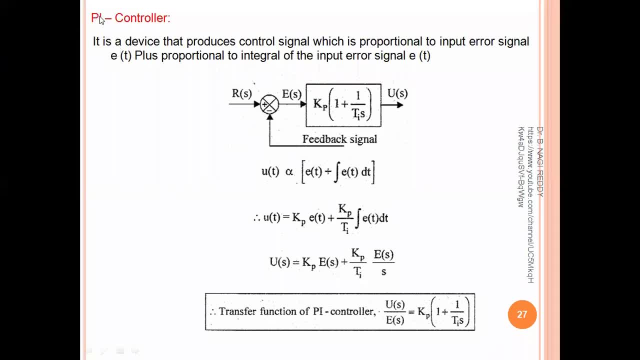 what we are doing here is we are adding p with i, so proportional controller and integral controller. so we are adding p and i. so that means we are having two signals. one is- you can see, it is the device that produces control signal, which is proportional to the input error signal. proportional to the input error signal. 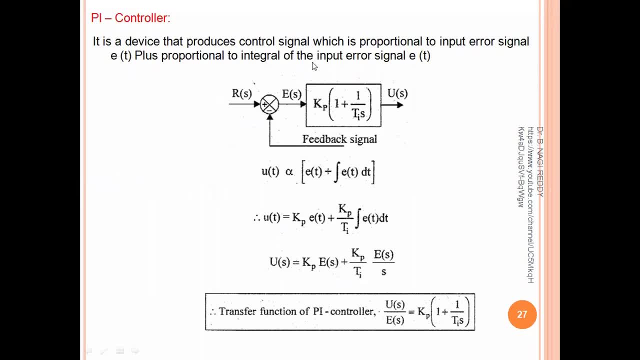 means p plus proportional to the integral of the input error signal, which is i. so this is i definition and this is p definition. if we, if you combine these two definitions, you will get the p- i controller definition simply, or from this definition we can write the mathematical representation, which is the. 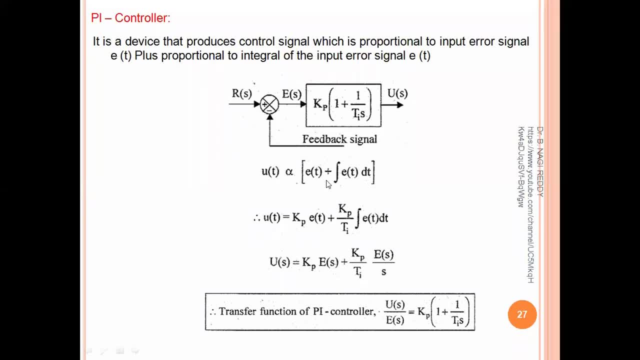 control signal. u of t is directly proportional to e of t plus integral of e of t. this integral of e of t is simply integration controller and here e of t, which is proportional controller. so if we add these two you'll get this equation. so in order to eliminate this proportionality, we use proportionality constant. 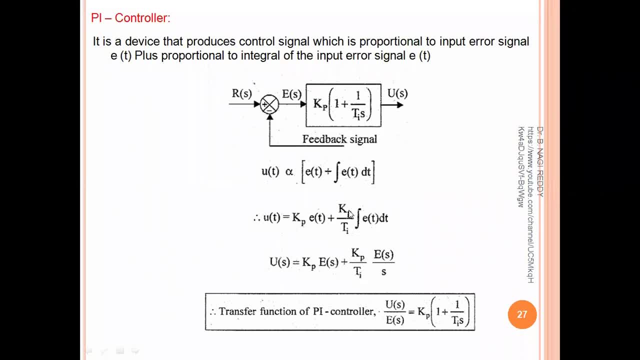 which is k p for proportional controller. here in the previous section i have told you in the play here we can use k i. k is the integral gain, but in the place of k? i we can write k p by t i in terms of k. i can be written in terms of k p. 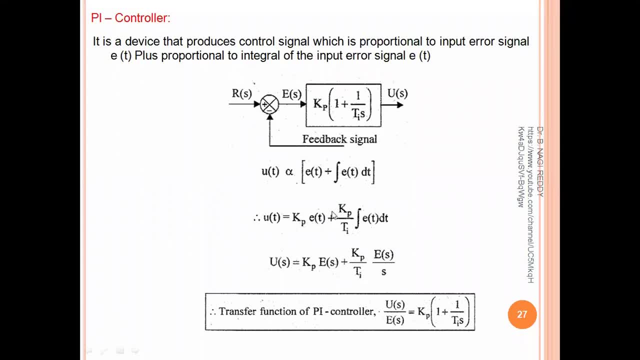 so k p by t i. because we can, we can take common k p right. so for the simplification purpose i have written this k i as k p by t i. now apply laplace transform to this equation, so we will get like this: so k p will be taken out and we can write the transfer function. 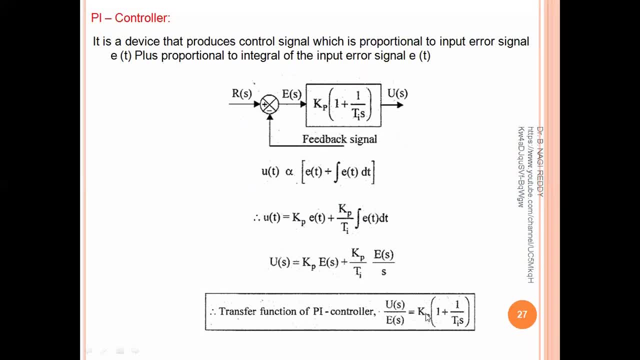 so we will get u of s by e, of s is equal to k- p into one plus one by TIS. So this will be the transfer function of this block. that's why, here you can see, the block is represented with this transfer function. So a simple addition of the proportional controller. 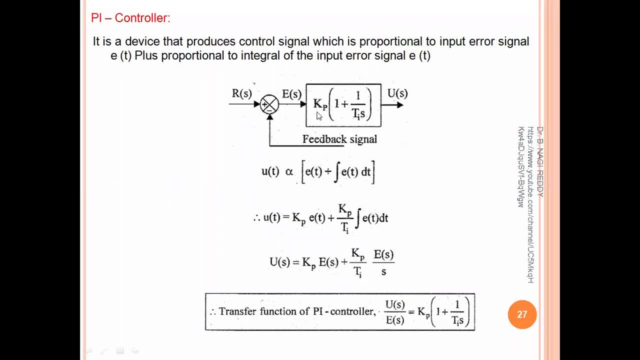 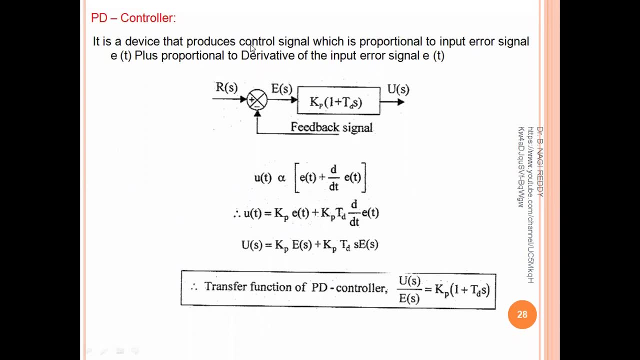 and the integral controller. that's it. okay, So this is PI controller. in the same manner, we can write for PD controller also, right? See that it produces the control signal, which is proportional to the input plus proportional to the derivative of the input, because this is TD, so D means derivative. 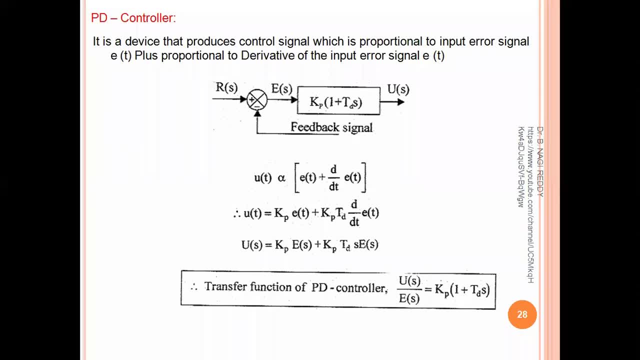 or a differentiative. So derivative is there. so what we write with the statement we will write: the output, which is U of T output, or simply control signal, is directly proportional to input error signal, which is ET and derivative of the error signal, which is D by DT of ET right. So to eliminate this we can simply: 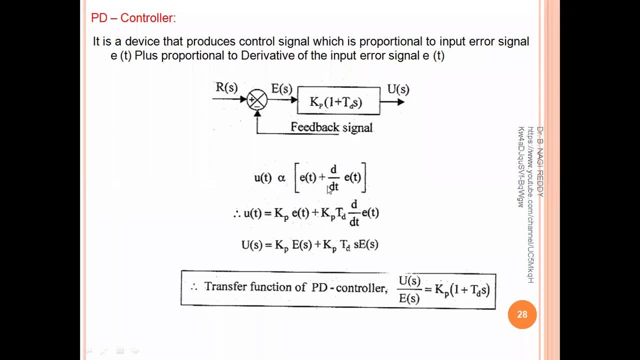 write KP here because this is proportionality term, and here you can write KD because derivative constant. but for simplification purpose this KD term can be written like this: KP into TD, where TD is the derivative time constant as we written in the integral controller. here also we can write KP into TD in. 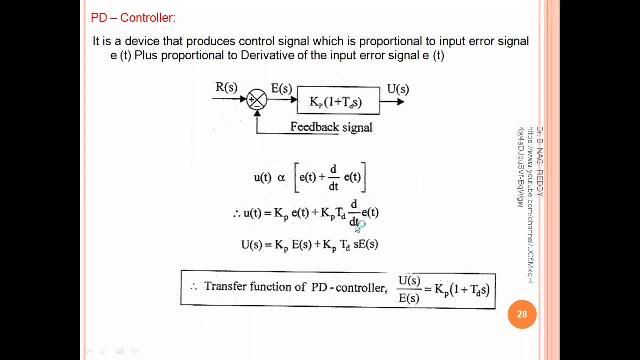 the similar manner. Now apply Laplace transform here. first order differentiation is there, So apply Laplace transform and write U of S by E of S, because U of S is our output of this controller. E of S is the input of controller. according to the Laplace transforms- sorry, according to the 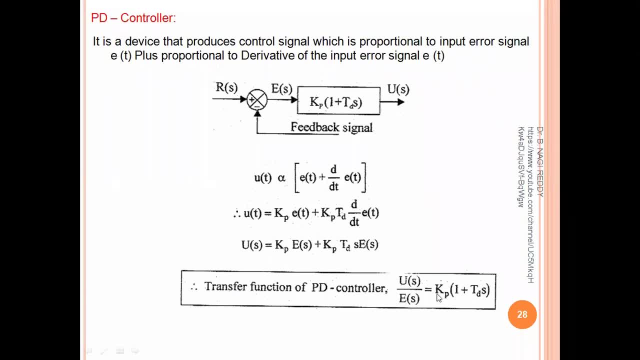 transfer function. we can write U of S by E of S from this. So then we write this equation: if you simplify we will get KP, because both in the both sections KP is constant. so take out the KP, so KP into 1, plus TD into S, So this is the gain of TD controller. now 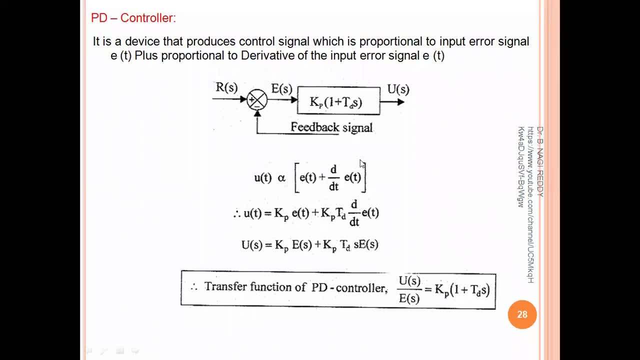 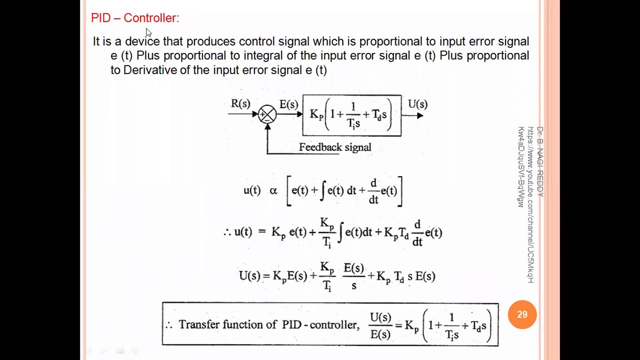 substitute. so gain means what? so we can write this value in the controller block like this. so we have seen pi, now pd and then pid controller in the similar manner. so what we do here, we will add proportional plus integral, plus derivative. this statement states the same, so proportional. 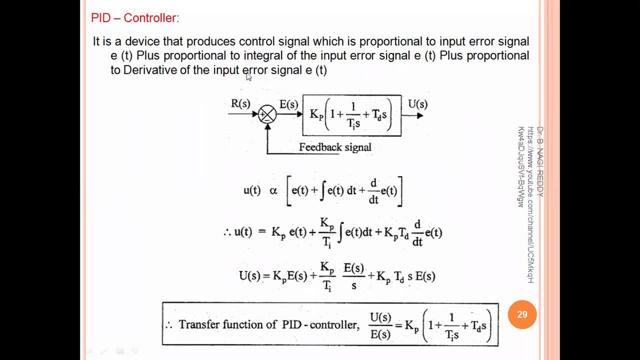 signal plus integral signal plus derivative signal, so these three signals can be combinedly added and generated. control signal is proportional to all these three. in order to eliminate this proportionality, so we can, we can write the gain constants, which is for proportional gain kp, for integral gain, kp by ti, for differential gain, kp, into td. right now for this equation: same. 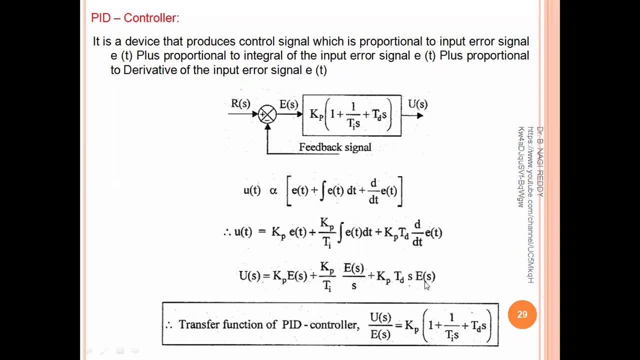 play laplace transforms, then we will get the. we will get this equation. take out kp as common, and es as es also common, and write u of s by e of s, because u of s is the output, e of s is the input. so from that we can write the transfer function. 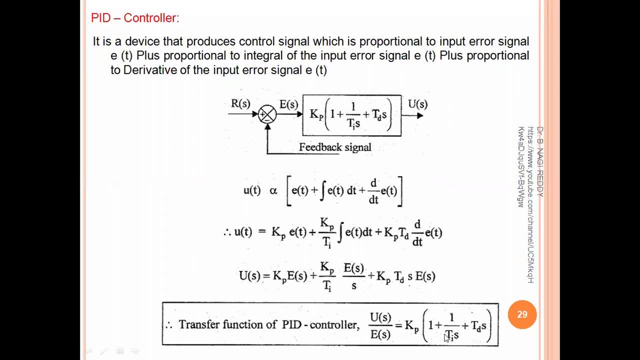 of the pid controller as kp into one plus one by tis plus tds. very, very simple, all the for all these six controllers. the process is very, very simple and same. okay, so this is how we can find out, or we can determine the transfer functions of these. 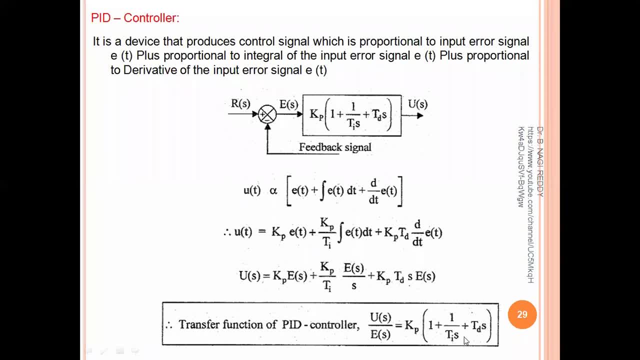 controllers. so these controllers having different terms- td, ti and kp. so in order to design a proper controller, we need to tune these values properly. so the kp value, ti value, td value. we need to choose these three values properly in order to choose a proper controller. so this PID controller accurately if this, if we tune this controller accurately. 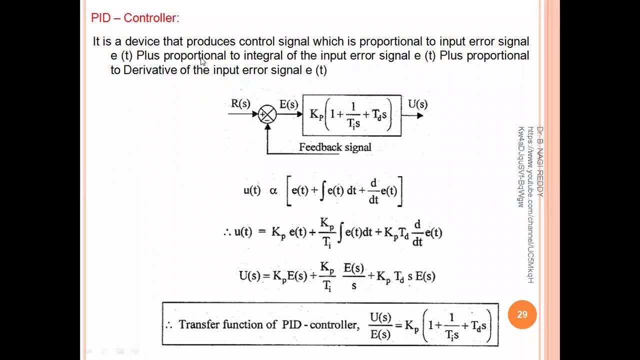 then the system will work very effectively. so the accuracy of this controller completely depends upon the values, what we choose, okay. so while designing the controller, we have to, we have to be careful about the accuracy of that particular. Tritium is radioactive but safe to handle as long as it's contained within its vials. Work carefully to avoid breaking the vials. If they do break, leave the area and ventilate it for a few hours to disperse the gas. Greetings, fellow nerds. 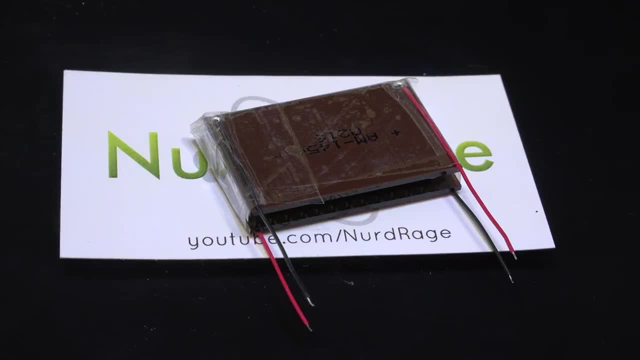 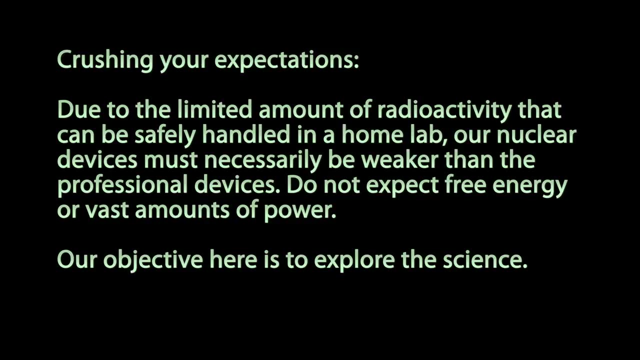 In this video we're going to make a very simple nuclear battery, But as usual, i need to crush your expectations. Due to the limited amount of radioactivity that can be safely handled in a home lab, our nuclear devices must necessarily be weaker than the professional devices. 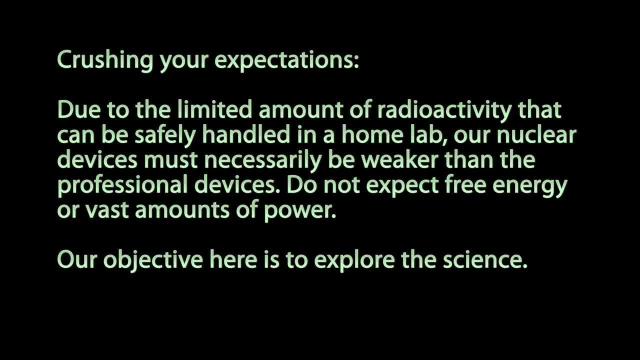 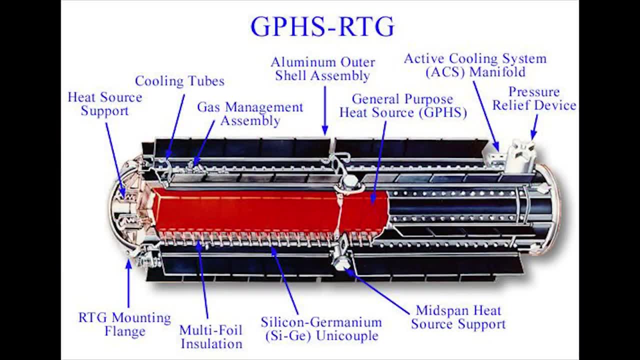 Do not expect free energy or vast amounts of power. Our objective here is to explore the science. As you may know, nuclear batteries or radioisotope thermoelectric generators are famously used on space probes due to their high power, density, reliability and longevity. They are also occasionally used in remote locations like unmanned lighthouses in the former soviet union. The military also uses such batteries for remote radar stations. Going to change the batteries on a regular basis was extremely costly, so nuclear batteries was thought to be a better option.